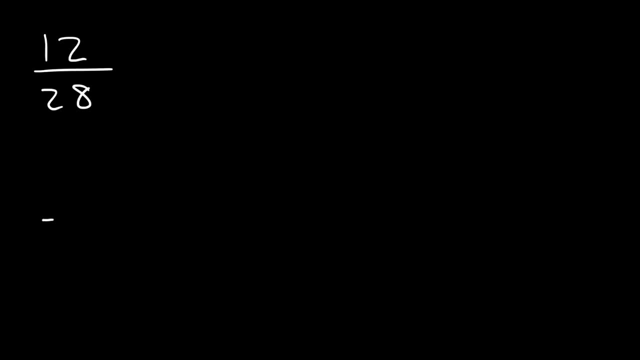 Reduce the fraction 12 over 28, and also 54 divided by 30.. Feel free to take a minute and work on these two examples. So what numbers can we break 12 into? Just like the last example, we can write it as 4 times 3.. Now what about 12?? What about 28?? 28 is 4 times 7.. So notice that we can cancel a 4 in this example. So 12 over 28 can be reduced to 3 over 7.. So that's a quick and simple way to reduce fractions. 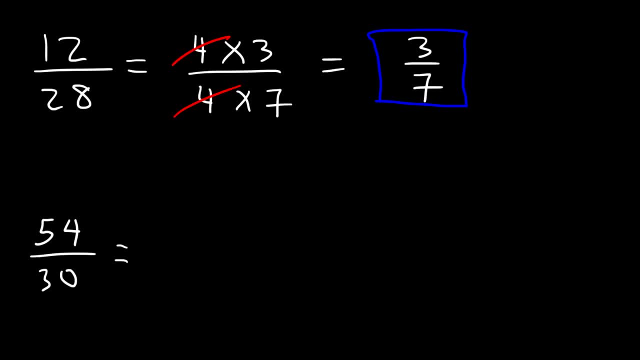 Try the next example: 54 and 30,. what numbers can we break down into? 54 is 9 times 6.. 30 is 5 times 6.. So in this example we can cancel a 6. And so we're left with 9 over 5.. 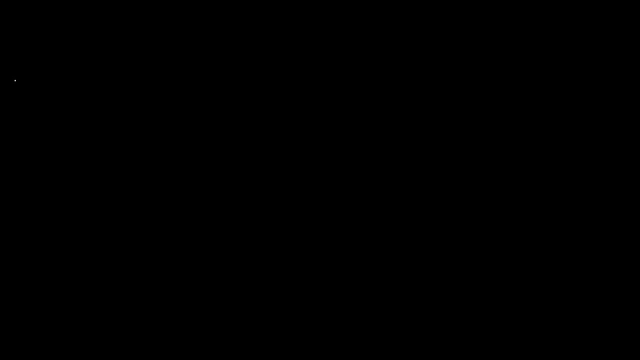 And that's the answer for the second example. Go ahead and try this one: 120 divided by 96.. So now we have some larger numbers to deal with. So what can we break down 120 into 120 is 12 times 10.. 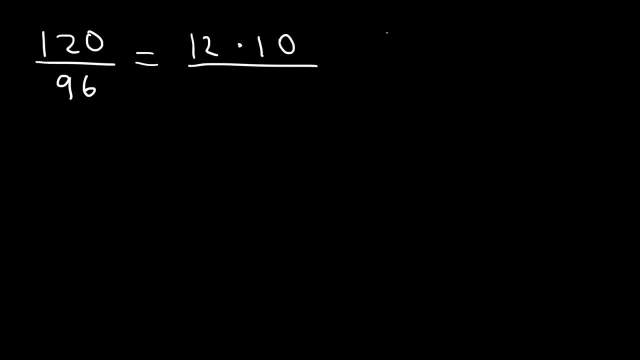 Now what about 96?? Well, we know 96 is an even number, So we can write it as 2 times 48.. Now 12,. we could break that down into smaller numbers: 4 times 3.. And 10 is 5 times 2.. 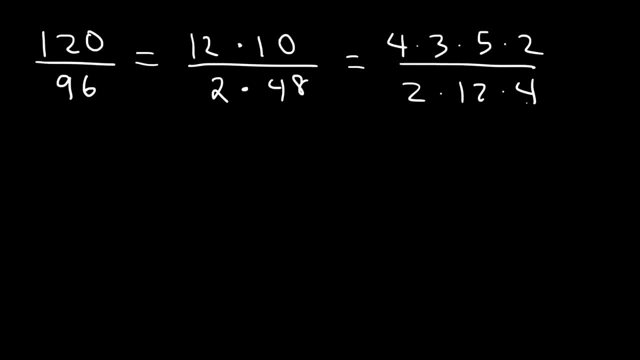 48 is 12 times 4.. So at this point we could cancel a 4 and we could cancel a 2.. So on top we have 3 times 5. And 12, we could break that into 3 times 4.. 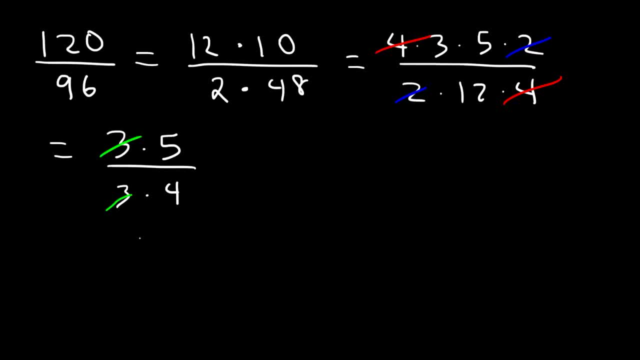 So we can go ahead and cancel a 3.. So therefore, the final answer in this example is 5 divided by 4.. So that's how you could simplify 120 over 96.. Let's try another example with a very large number. 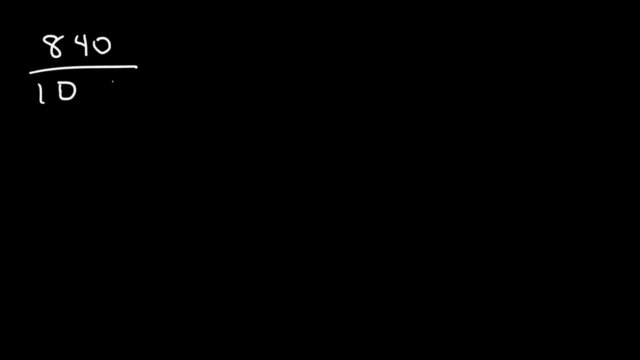 840 divided by 10,000, I mean 1,050.. So take a minute and try that one. So 840, we can write it as 84 times 10.. 1,050 is basically 105 times 10.. 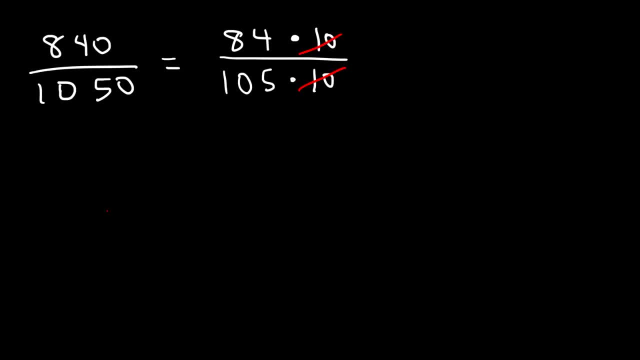 So we can get rid of the 10.. Now 84, what numbers go into 84?? Well, we know it's an even number, So we could divide it by 2.. 84 divided by 2 is 42. So we can write it as 2 times 42.. 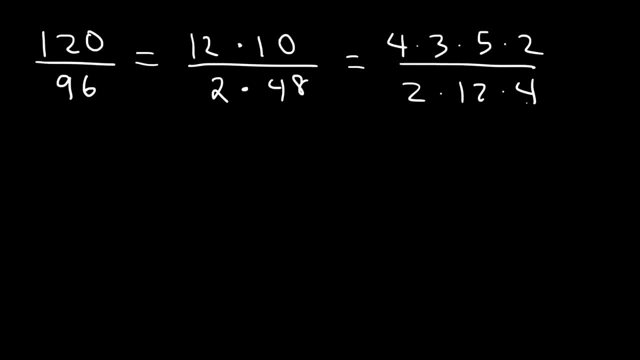 48 is 12 times 4.. So at this point we could cancel a 4 and we could cancel a 2.. So on top we have 3 times 5. And 12, we could break that into 3 times 4.. 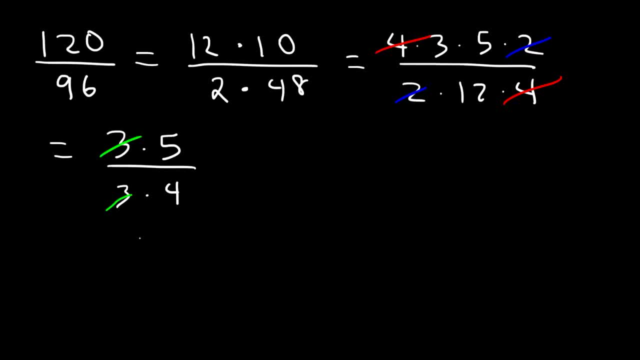 So we can go ahead and cancel a 3.. So therefore, the final answer in this example is 5 divided by 4.. So that's how you could simplify 120 over 96.. Let's try another example with a very large number. 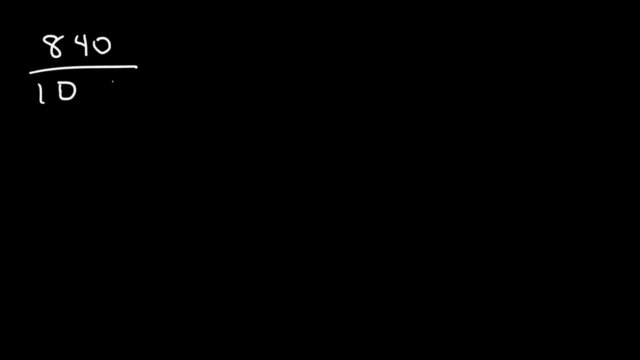 840 divided by 10,000, I mean 1,050.. So take a minute and try that one. So 840, we can write it as 84 times 10.. 1,050 is basically 105 times 10.. 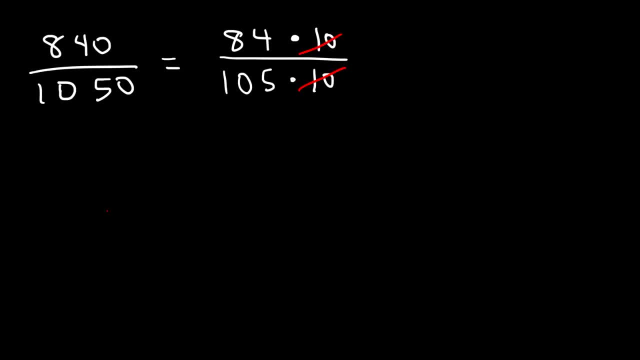 So we can get rid of the 10.. Now 84, what numbers go into 84?? Well, we know it's an even number, So we could divide it by 2.. 84 divided by 2 is 42. So we can write it as 2 times 42.. 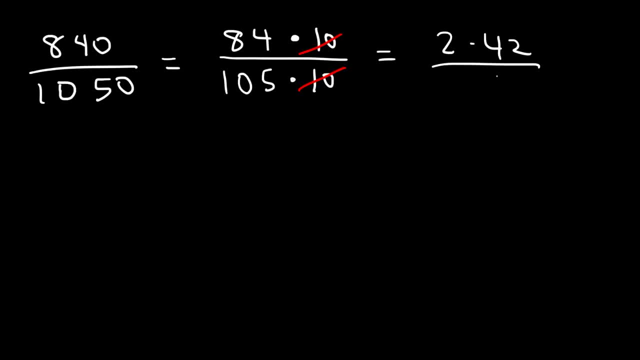 105 is divisible by 5, since it ends in 5. So this is 5 over 21.. Now 42 is 7 times 6.. 21 is 7 times 3.. So at this point we can get rid of a 7.. 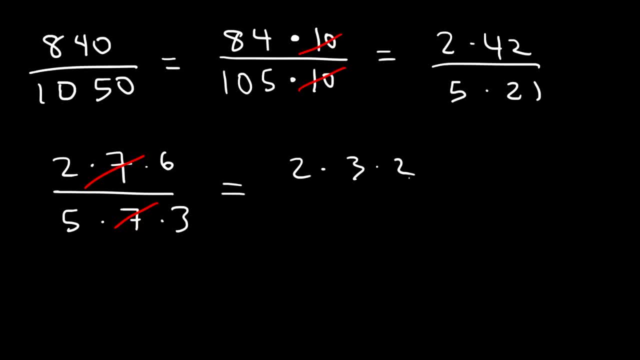 And 6 is 3 times 2.. So now we can get rid of a 3.. So the final answer for this example is 4 divided by 5.. Now let's try an example that has variables x to the 4th divided by x. 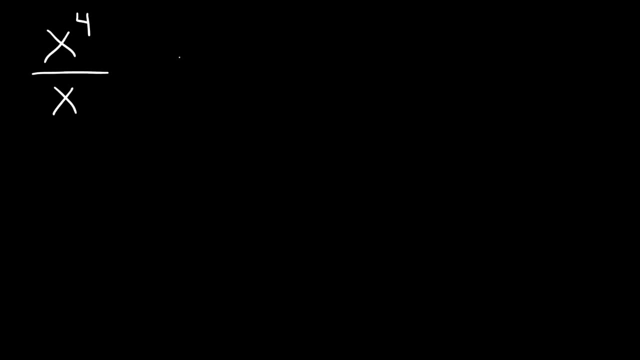 So how can we simplify this algebraic fraction? Well, what we could do is factor x to the 4th. x to the 4th is basically 4 x variables multiplied to each other. Now what we can do is cancel one of the x variables. 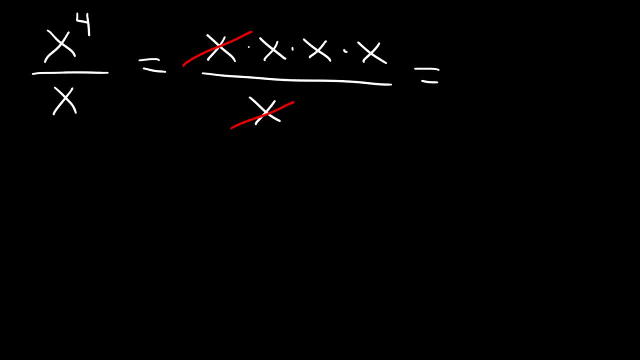 on the top and on the bottom. So notice that we have 3 x variables left over on top. Therefore, this is x cubed over 1, or simply x cubed. So that's the answer for this example. Here's another one that we could work on. 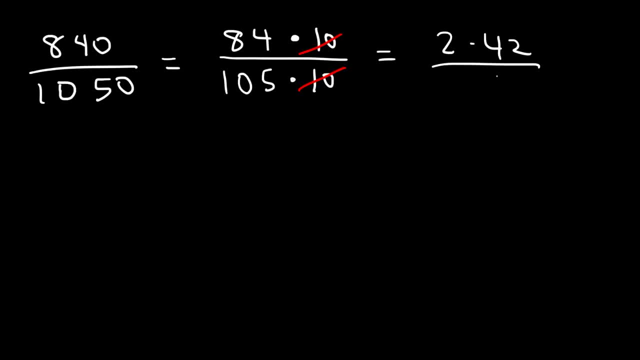 105 is divisible by 5, since it ends in 5. So this is 5 over 21.. Now 42 is 7 times 6.. 21 is 7 times 3.. So at this point we can get rid of a 7.. 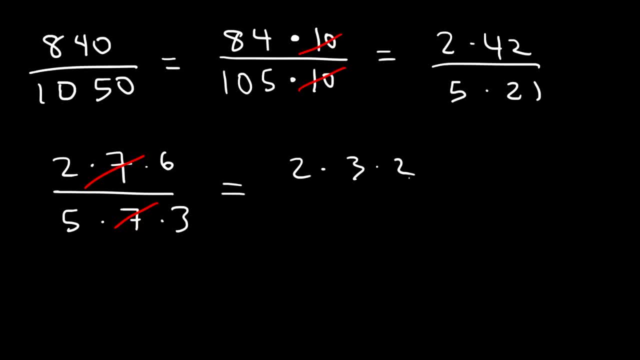 And 6 is 3 times 2.. So now we can get rid of a 3.. So the final answer for this example is 4 divided by 5.. Now let's try an example that has variables x to the 4th divided by x. 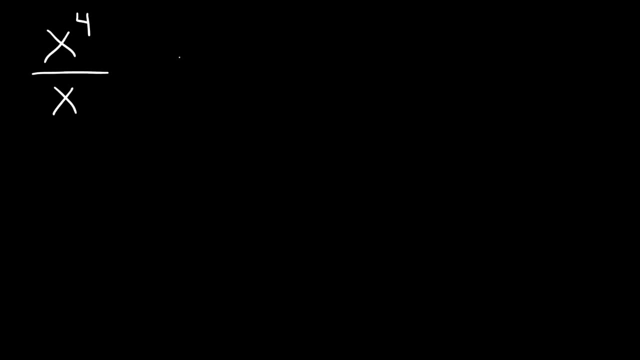 So how can we simplify this algebraic fraction? Well, what we could do is factor x to the 4th. x to the 4th is basically 4 x variables multiplied to each other. Now what we can do is cancel one of the x variables. 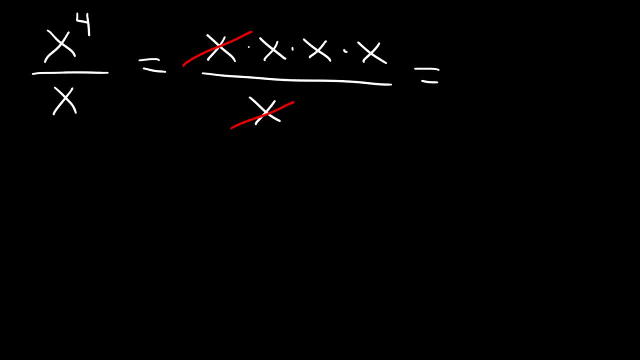 on the top and on the bottom. So notice that we have 3 x variables left over on top. Therefore, this is x cubed over 1, or simply x cubed. So that's the answer for this example. Here's another one that we could work on. 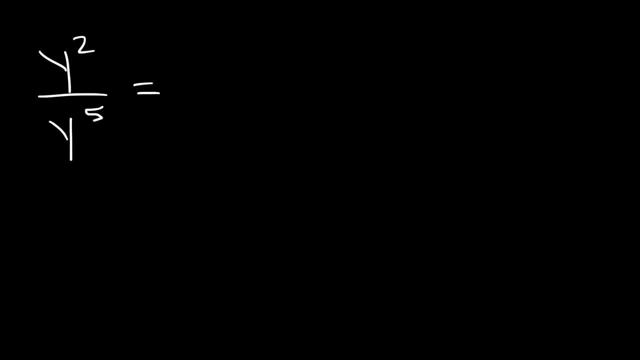 y squared divided by y to the 5th. What do you think the answer is For this problem? based on the last example that you saw, y squared is y times y And y to the 5th. power is basically 5 y variables multiplied to each other. 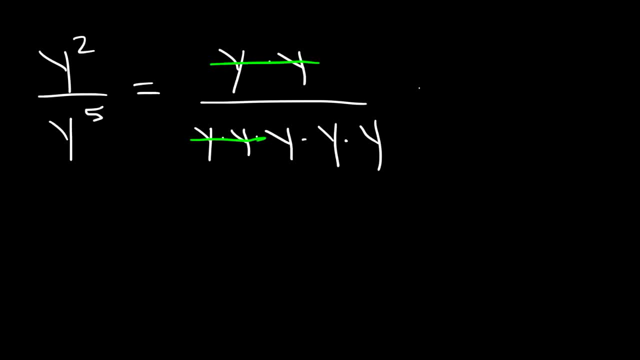 So we can cancel 2 of them on each side of the fraction. So now we have none on top, So we're just going to write 1.. y divided by y is 1. And on the bottom there are 3 y variables left over. 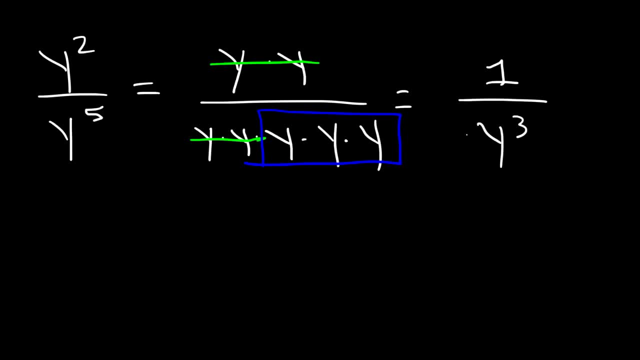 So it's going to be y cubed on the bottom. So this is the answer: 1 divided by y cubed. Here's another example: 9 x squared, divided by 15. x to the 5th. Go ahead and try that one. 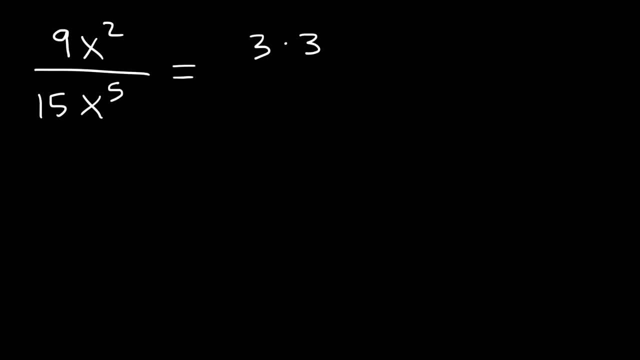 9, we can write it as 3 times 3.. x squared is x times x, 15 is 5 times 3.. y to the 5th power is 5 x variables multiplied to each other. So we could cancel a 3 in this example. 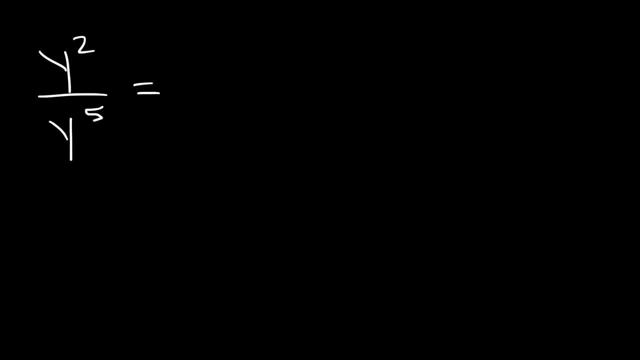 y squared divided by y to the 5th. What do you think the answer is For this problem? based on the last example that you saw, y squared is y times y And y to the 5th. power is basically 5 y variables multiplied to each other. 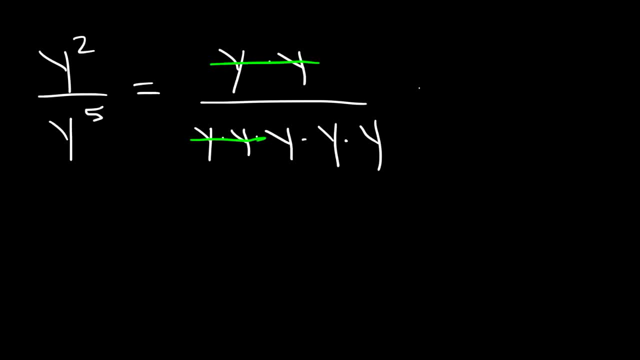 So we can cancel 2 of them on each side of the fraction. So now we have none on top, So we're just going to write 1.. y divided by y is 1. And on the bottom there are 3 y variables left over. 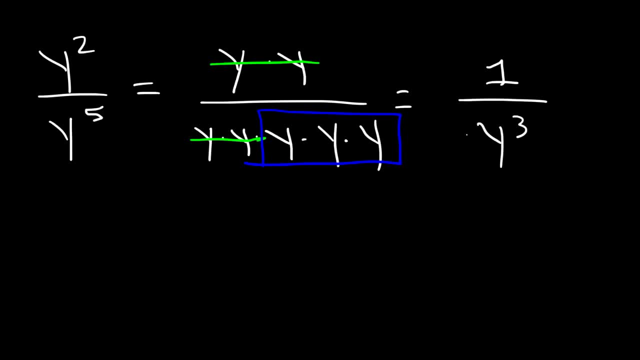 So it's going to be y cubed on the bottom. So this is the answer: 1 divided by y cubed. Here's another example: 9 x squared, divided by 15. x to the 5th. Go ahead and try that one. 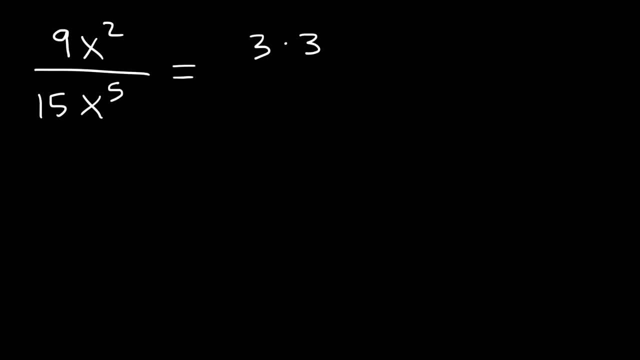 9, we can write it as 3 times 3.. x squared is x times x, 15 is 5 times 3.. y to the 5th power is 5 x variables multiplied to each other. So we could cancel a 3 in this example. 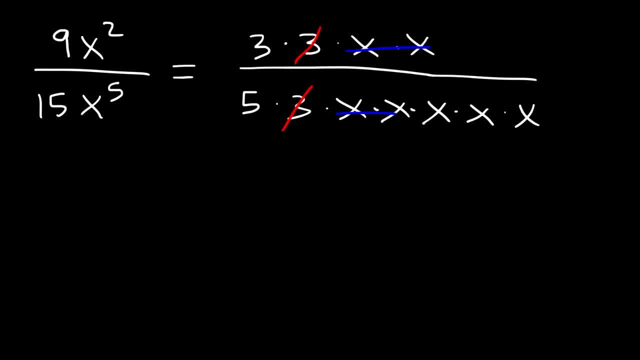 And we can cancel 2 of the x variables on top and on the bottom of the fraction. So all we have on the top of the fraction is a 3. On the bottom we have a 5. And we have 3 x variables. 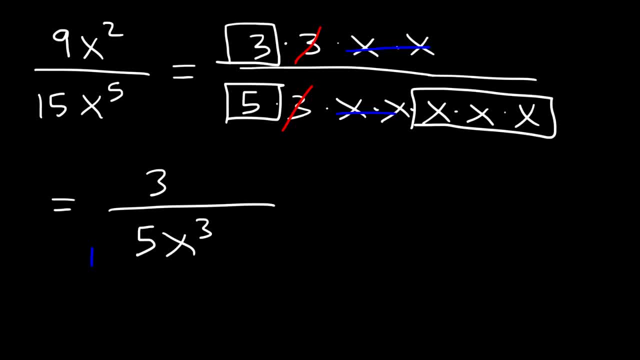 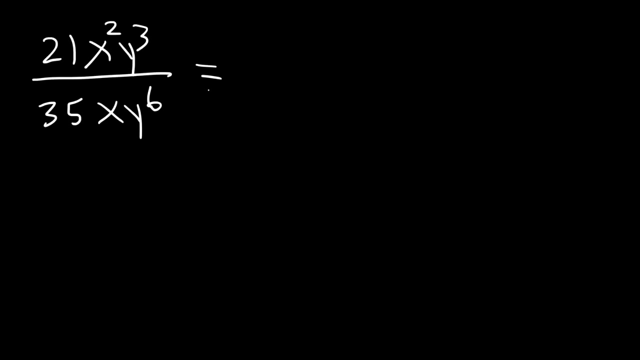 So the answer is 3 divided by 5 x cubed. Let's try this one: 21 x squared y cubed divided by 35 x y to the 6th. So what do you think we need to do? 21 and 35 both contain a 7.. 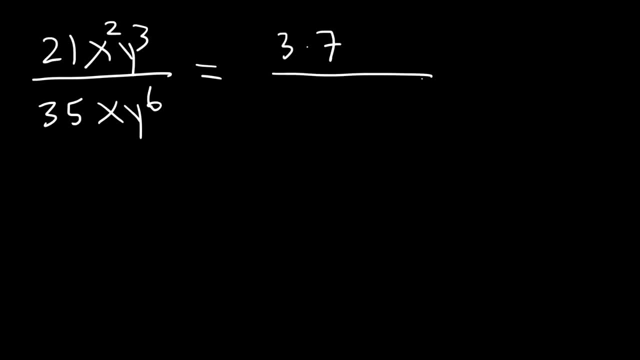 21 is 3 times 7.. And 35 is 5 times 7.. x squared is x times x, y cubed is just y times x, And then we have an x on the bottom and y to the 6 on the bottom as well. 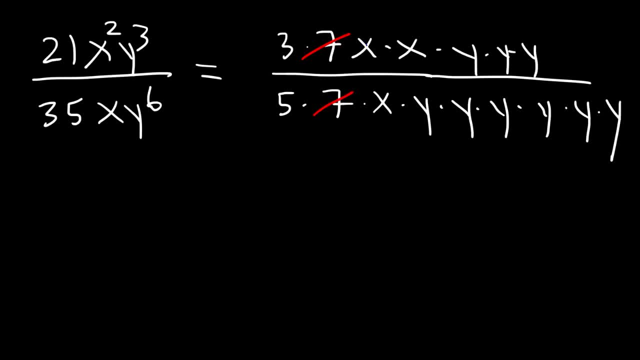 So we can cancel a 7,, an x and we can cancel 3 y variables. So on the numerator we're left with 3 x And on the bottom we have a 5. And just 3 y variables. 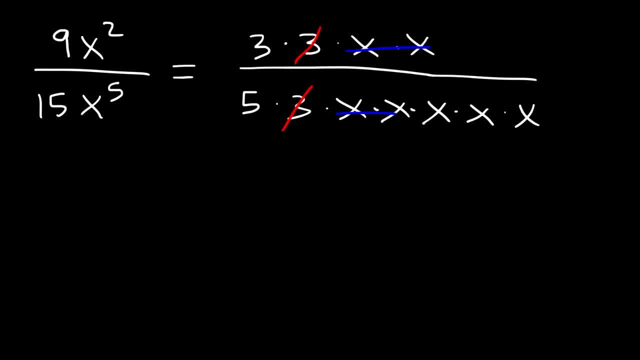 And we can cancel 2 of the x variables on top and on the bottom of the fraction. So all we have on the top of the fraction is a 3. On the bottom we have a 5. And we have 3 x variables. 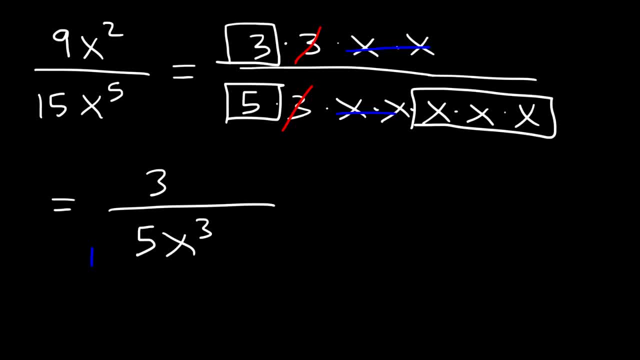 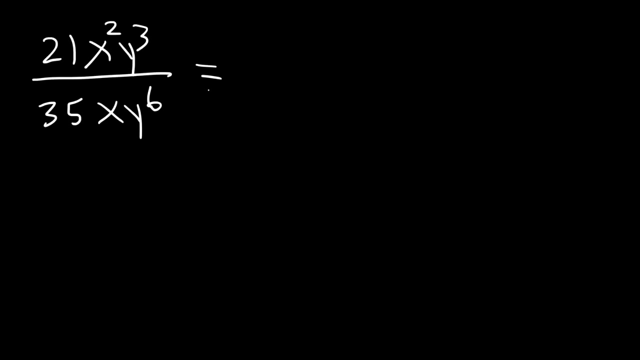 So the answer is 3 divided by 5 x cubed. Let's try this one: 21 x squared y cubed divided by 35 x y to the 6th. So what do you think we need to do? 21 and 35 both contain a 7.. 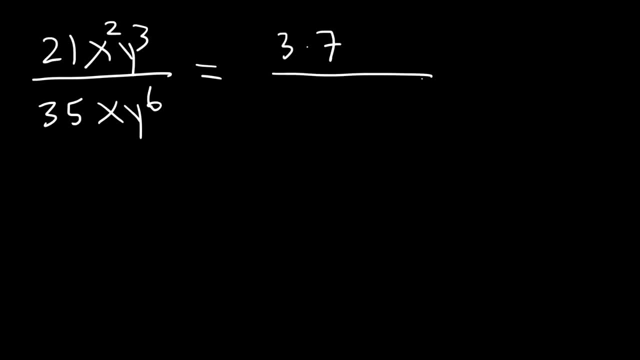 21 is 3 times 7.. And 35 is 5 times 7.. x squared is x times x, y cubed is just y times x, And then we have an x on the bottom and y to the 6 on the bottom as well. 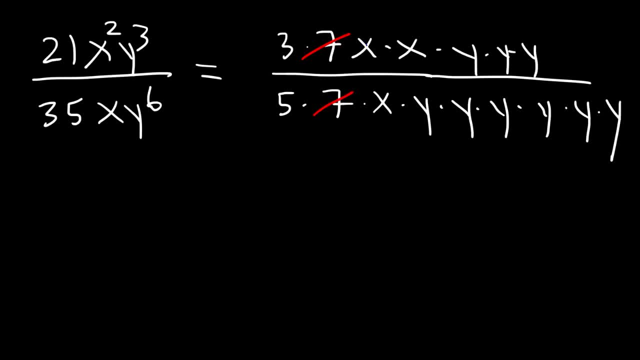 So we can cancel a 7,, an x and we can cancel 3 y variables. So on the numerator we're left with 3 x And on the bottom we have a 5. And just 3 y variables. 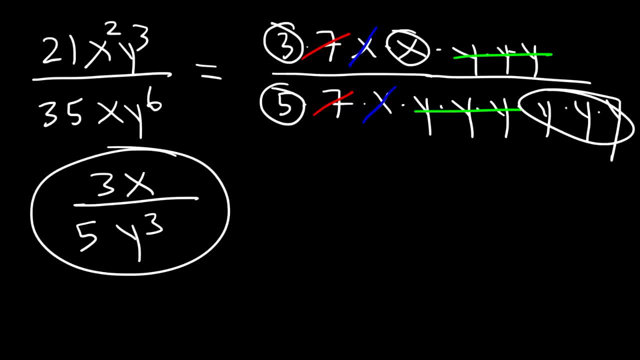 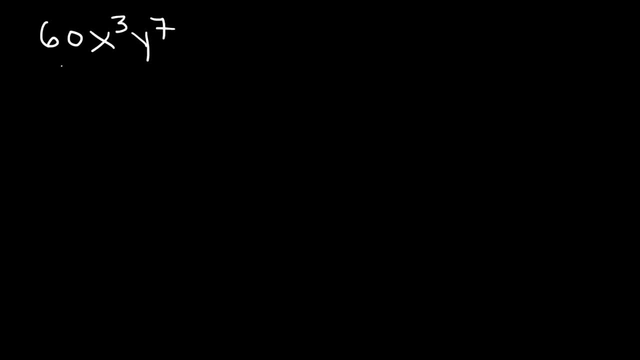 So the answer is 3 x over 5 y cubed. For the sake of practice, let's try one more: 60 x cubed y to the 7th, divided by 48. x to the 5th, y to the 4th. 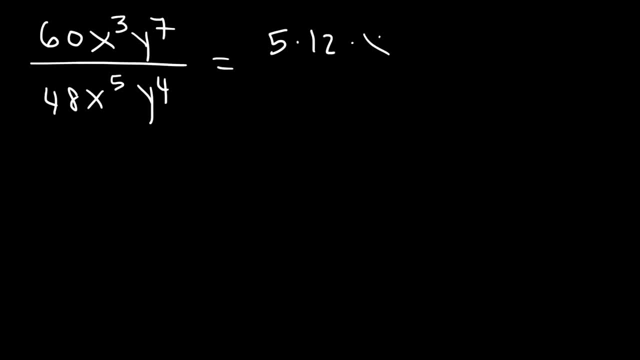 60 is basically 5 times 12.. And then we have x cubed and y to the 7th. So we have 7 y variables, And I'm almost out of space. 48 is 4 times 12.. And then we have x to the 5th and y to the 4th. 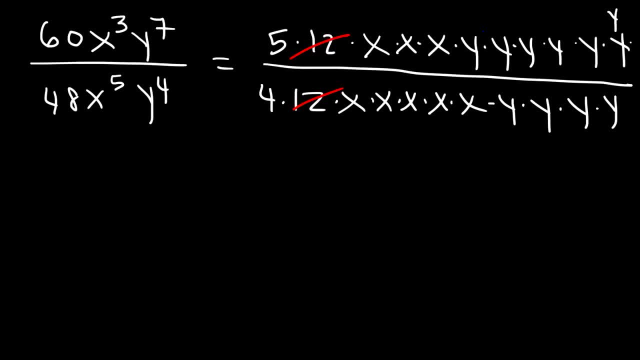 So we can cancel a 12. And we can cancel 3 x variables on both sides And we can get rid of 4 y variables. So on the numerator we're left with 3 y variables. So that's going to be y cubed. 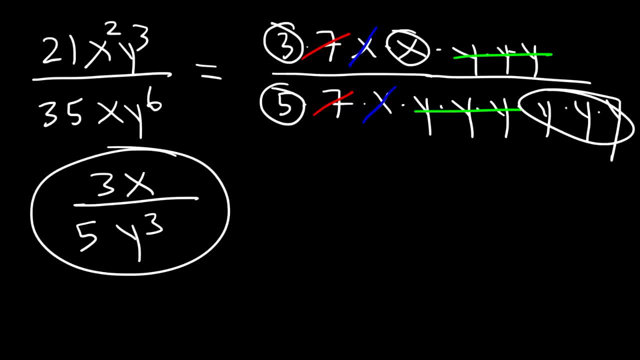 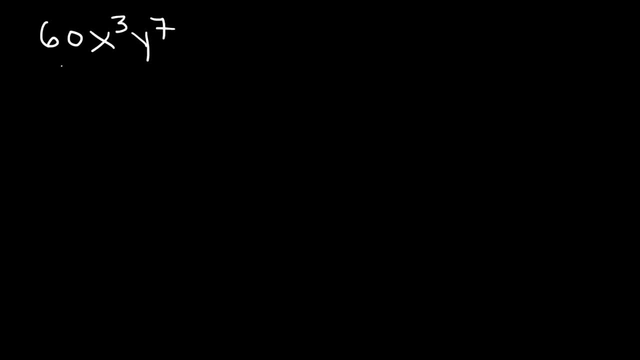 So the answer is 3 x over 5 y cubed. For the sake of practice, let's try one more: 60 x cubed y to the 7th, divided by 48. x to the 5th, y to the 4th. 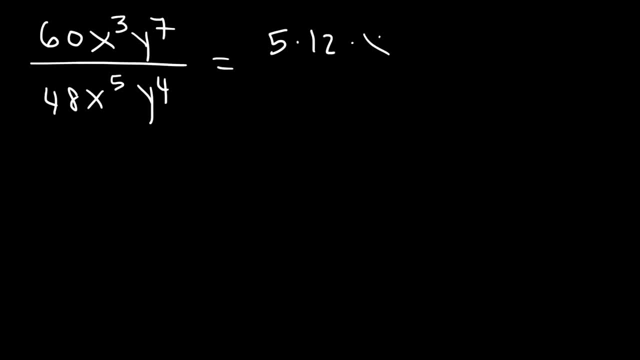 60 is basically 5 times 12.. And then we have x cubed and y to the 7th. So we have 7 y variables, And I'm almost out of space. 48 is 4 times 12.. And then we have x to the 5th and y to the 4th. 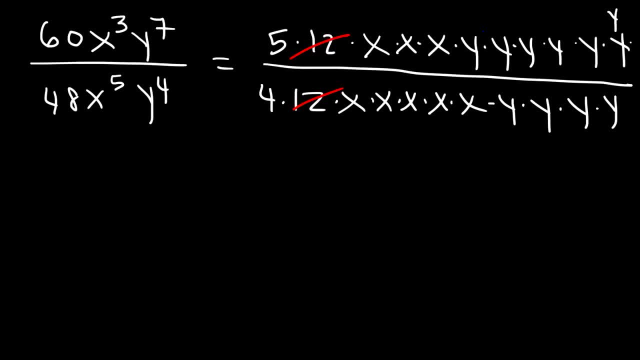 So we can cancel a 12. And we can cancel 3 x variables on both sides And we can get rid of 4 y variables. So on the numerator we're left with 3 y variables. So that's going to be y cubed. 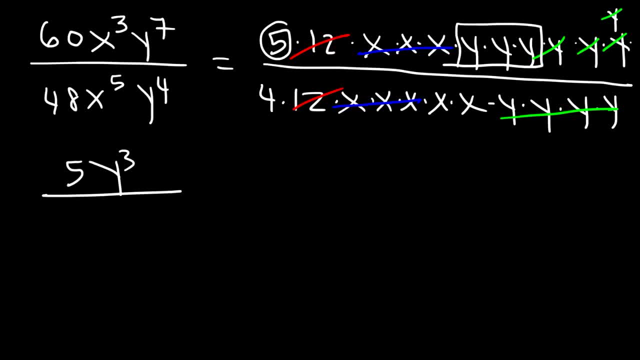 And we still have a 5 on top, So 5 y cubed. There's a 4 on the bottom And just 2 x variables, So 4 x squared. So 5 y cubed divided by 4 x squared is the final answer. 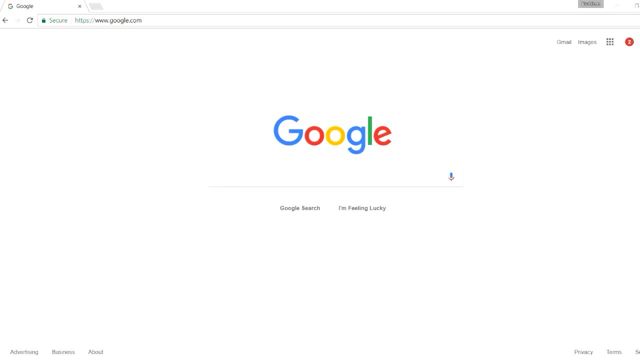 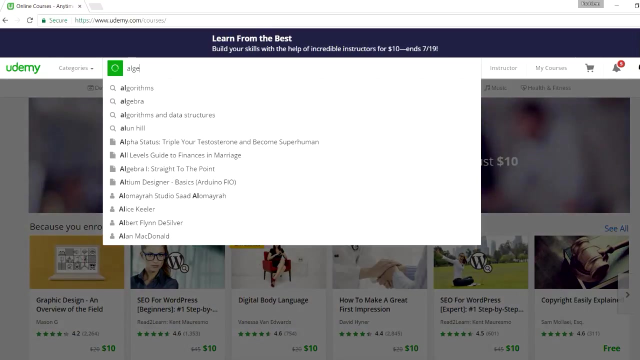 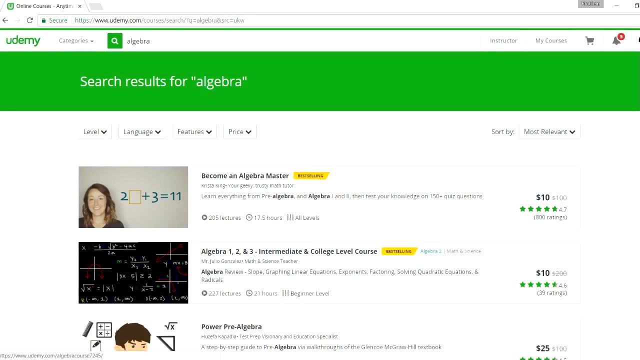 Now I want to show you one of my algebra courses that might be useful to you if you ever need it. So go to udemycom Now in the search box just type in algebra And it should come up. So it's the one with the image with the black background. 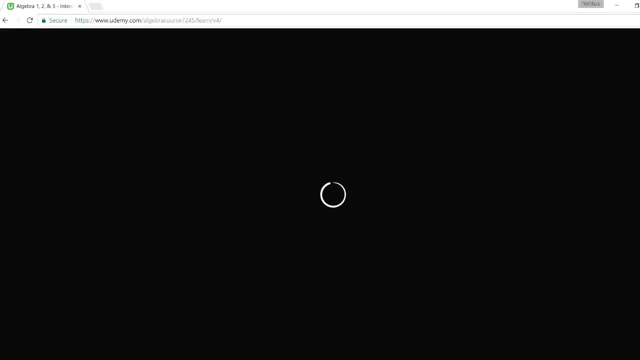 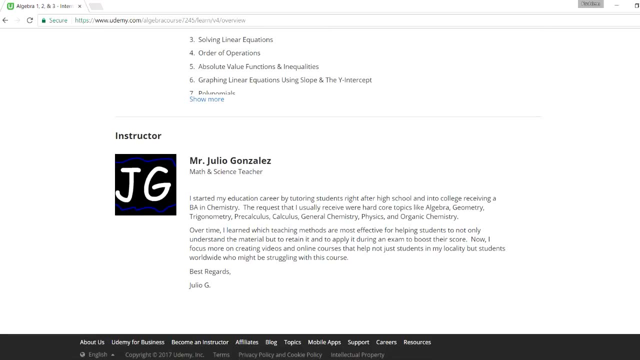 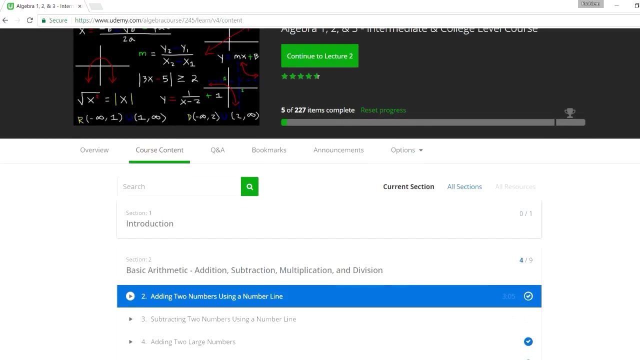 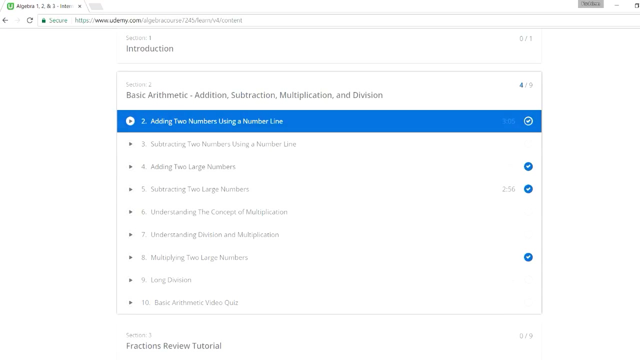 So if you select that option and if you decide to go to course content, you can see what's in this particular course. So the first section, basic arithmetic. for those of you who want to focus on addition, subtraction, multiplication and division: 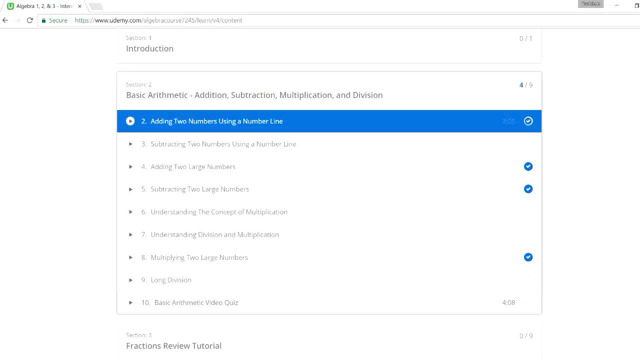 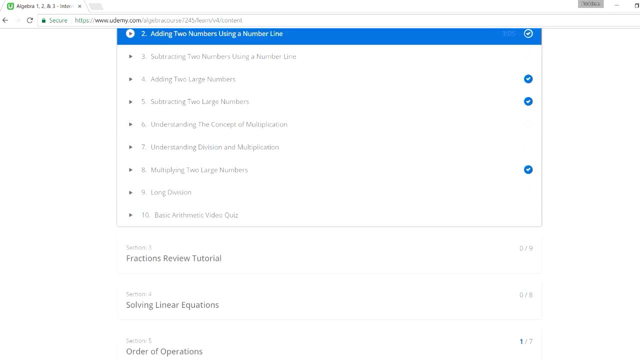 And it has a video quiz at the end. It's a multiple choice video quiz. You can pause it, work on the problems and see the solutions. It covers long division, multiplying two large numbers and things like that. The next tutorial is on fractions. 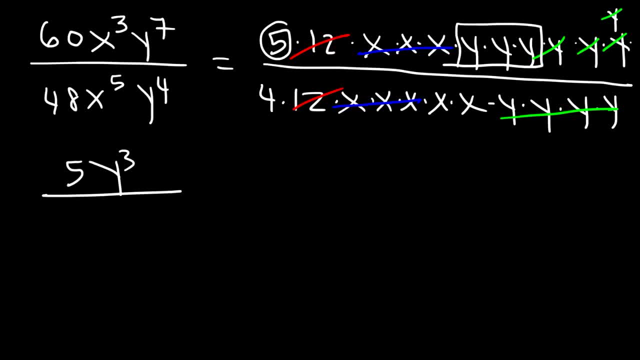 And we still have a 5 on top, So 5 y cubed. There's a 4 on the bottom And just 2 x variables, So 4 x squared. So 5 y cubed divided by 4 x squared is the final answer. 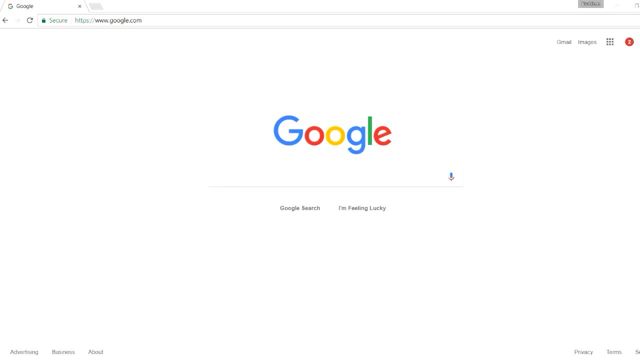 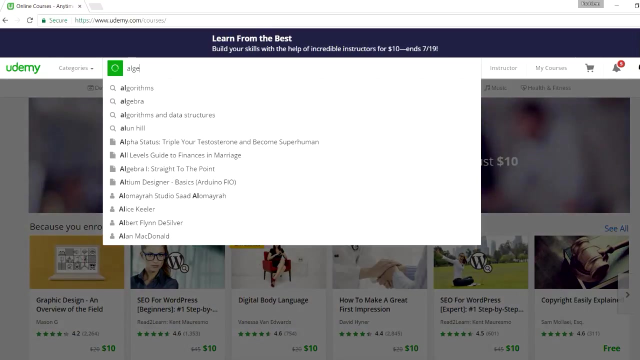 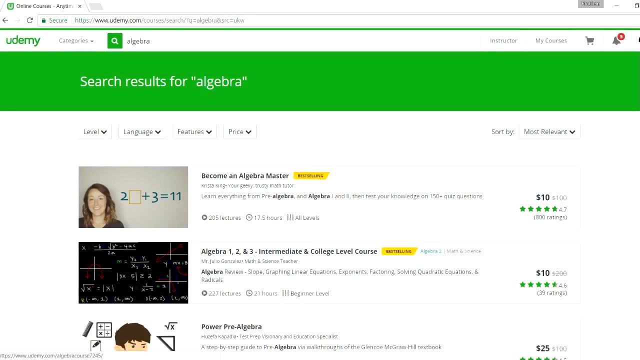 Now I want to show you one of my algebra courses that might be useful to you if you ever need it. So go to udemycom Now in the search box just type in algebra And it should come up. So it's the one with the image with the black background. 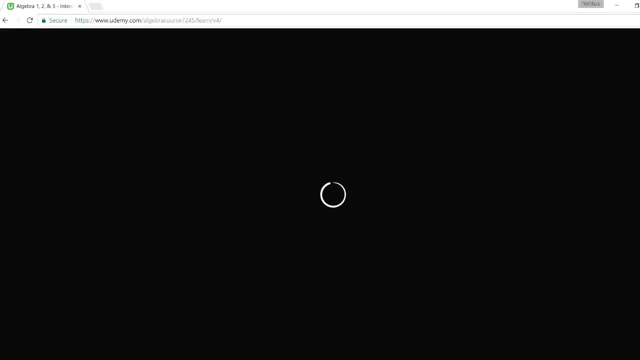 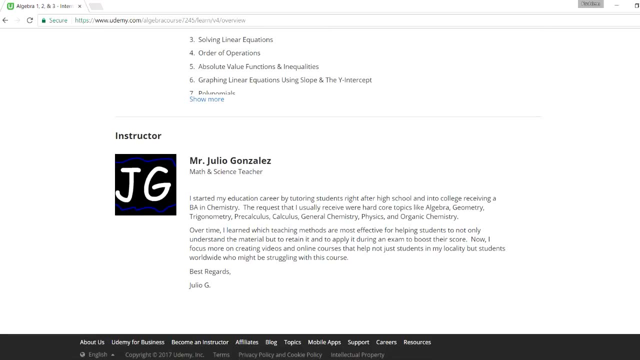 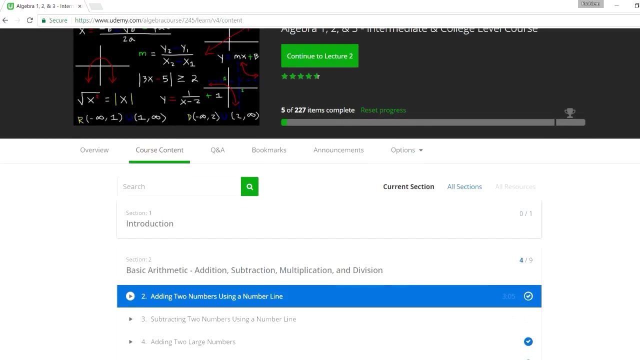 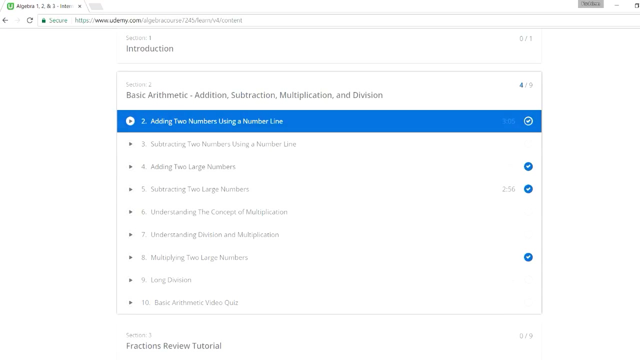 So if you select that option and if you decide to go to course content, you can see what's in this particular course. So the first section, basic arithmetic. for those of you who want to focus on addition, subtraction, multiplication and division: 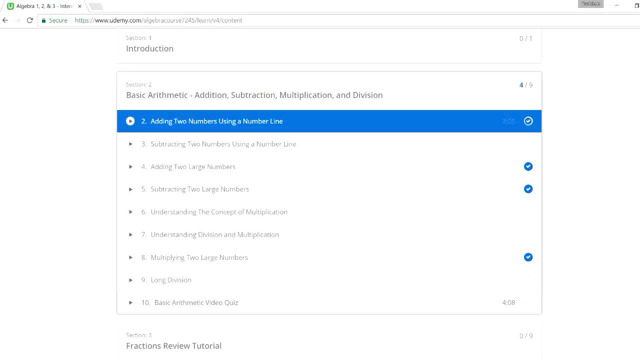 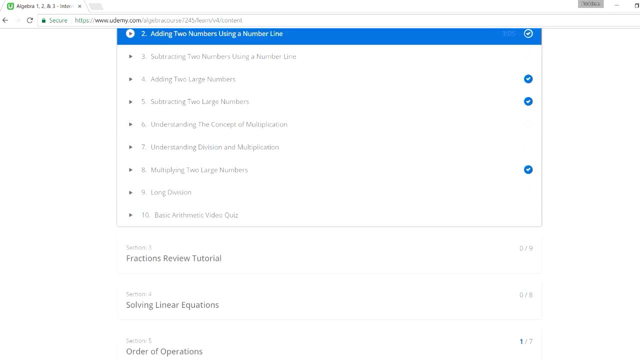 And it has a video quiz at the end. It's a multiple choice video quiz. You can pause it, work on the problems and see the solutions. It covers long division, multiplying two large numbers and things like that. The next tutorial is on fractions. 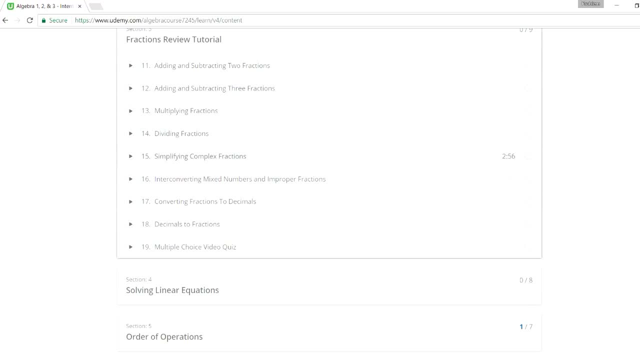 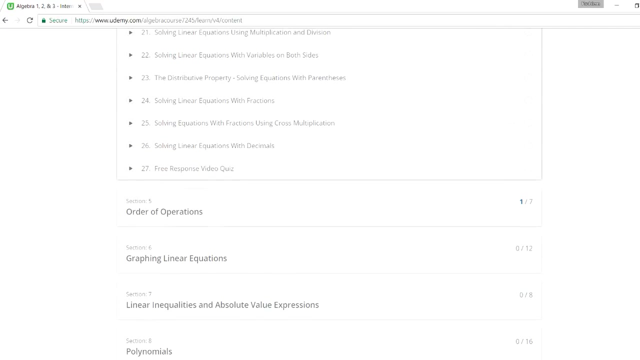 Add-in: subtracting fractions, multiplying and dividing fractions, converting fractions into decimals and so forth, So you can also take a look at that. Next, solving linear equations, which we covered, And just more examples if you need more help with that. 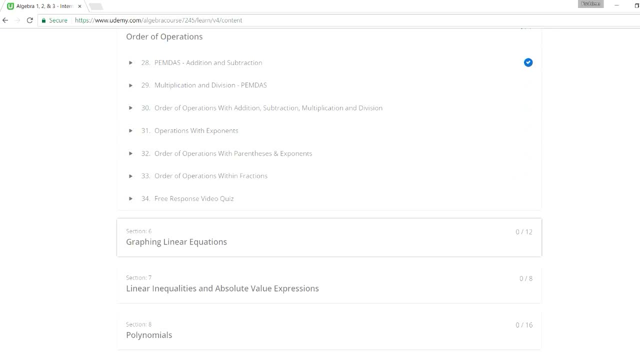 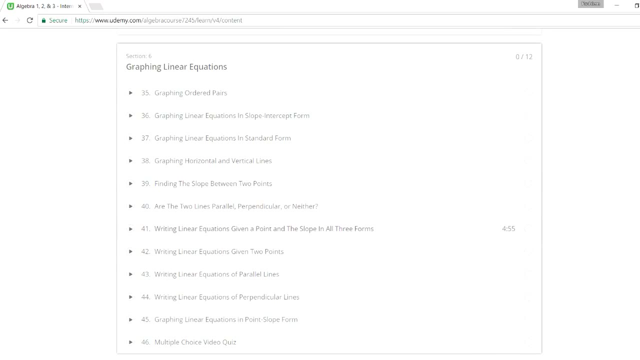 The next topic, order of operations, which is also useful: Graphing linear equations. You need to know how to calculate the slope, You need to be familiar with the slope intercept form, standing form and just how to tell if lines are parallel, perpendicular and so forth. 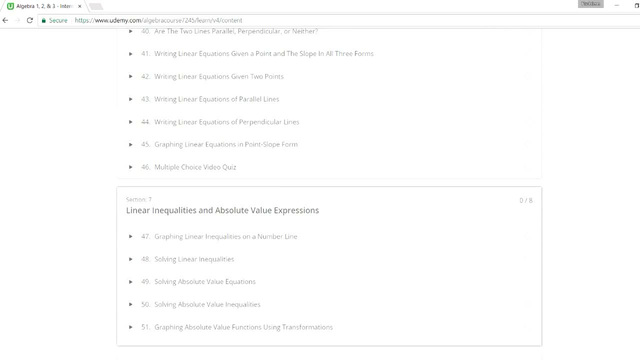 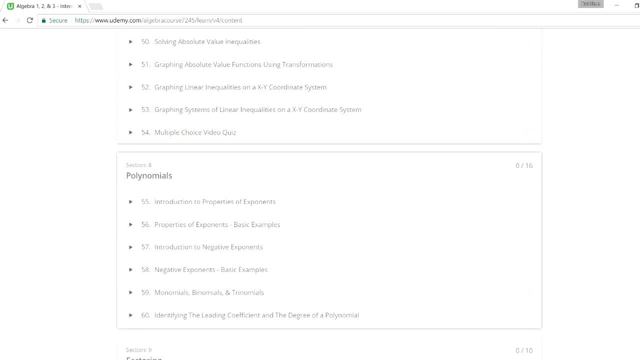 And there's a quiz that goes with that as well. The next topic is on inequalities and absolute value expressions, which are also seen in a typical algebra course, And then we have polynomials, And that's a long section, And then factoring. 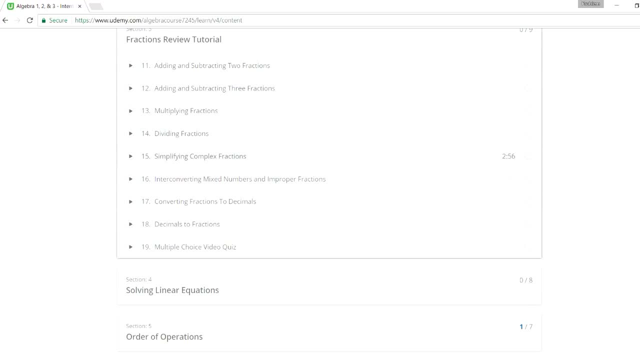 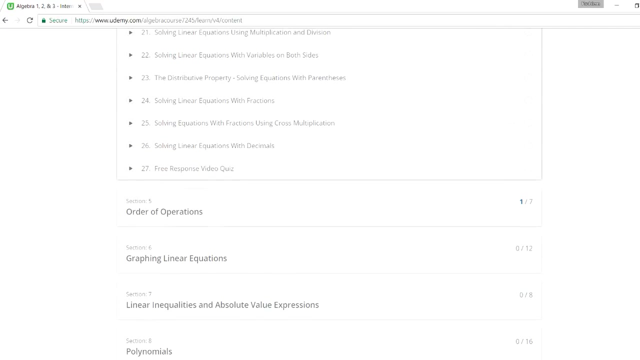 Add-in: subtracting fractions, multiplying and dividing fractions, converting fractions into decimals and so forth, So you can also take a look at that. Next, solving linear equations, which we covered, And just more examples if you need more help with that. 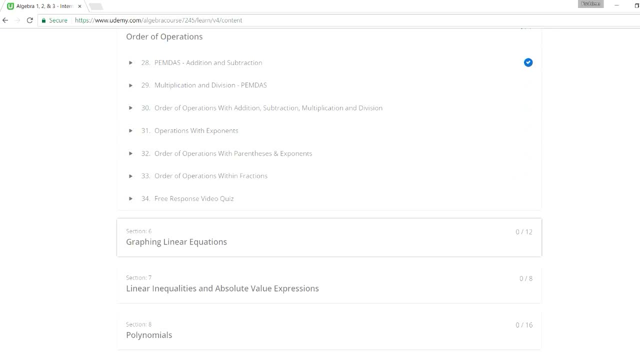 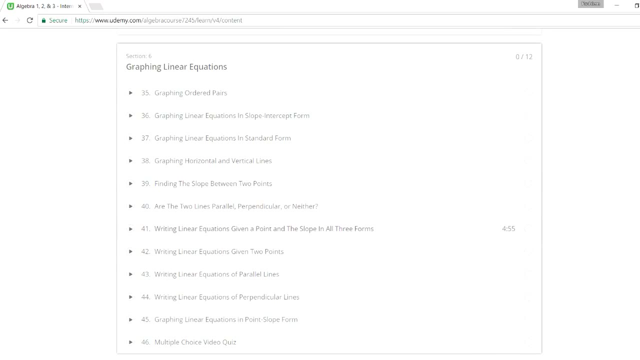 The next topic, order of operations, which is also useful: Graphing linear equations. You need to know how to calculate the slope, You need to be familiar with the slope intercept form, standing form and just how to tell if lines are parallel, perpendicular and so forth. 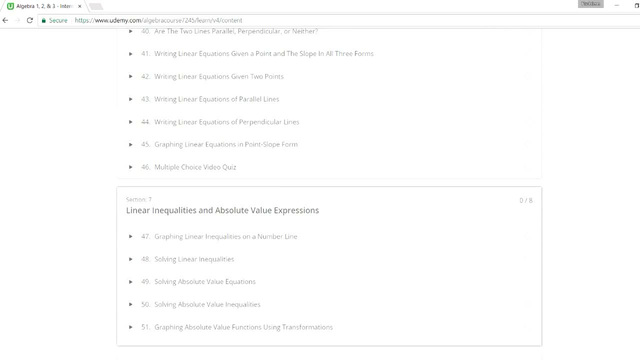 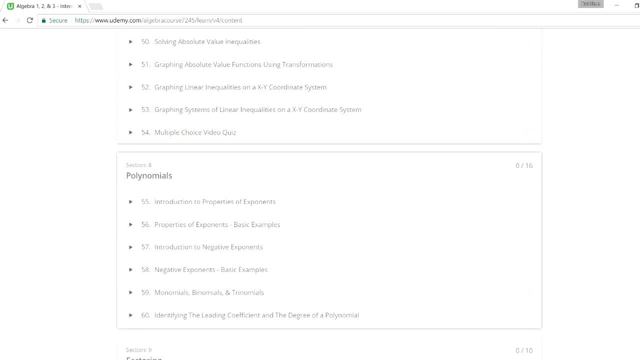 And there's a quiz that goes with that as well. The next topic is on inequalities and absolute value expressions, which are also seen in a typical algebra course, And then we have polynomials, And that's a long section, And then factoring. 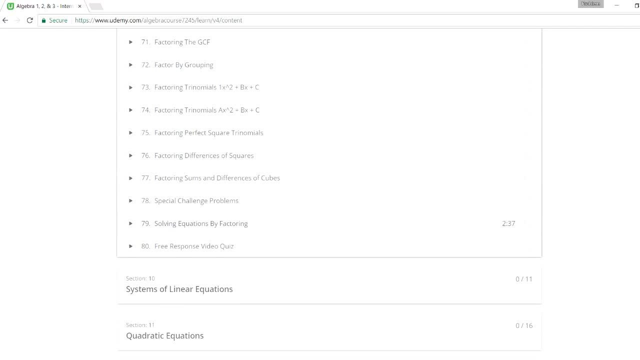 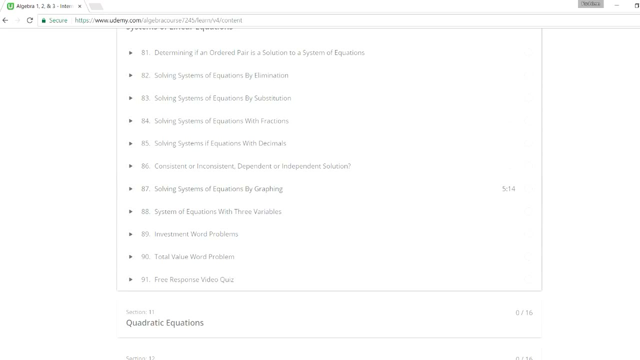 That's another topic you need to master. And then system of equations. You can solve it by elimination substitution. There's also word problems as well. Sometimes you've got to solve equations with three variables- x, y and z. So that could be helpful. 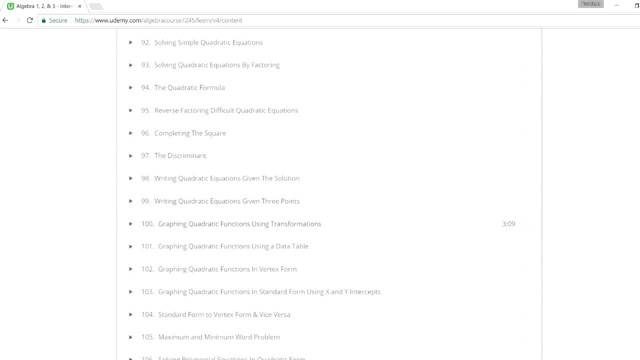 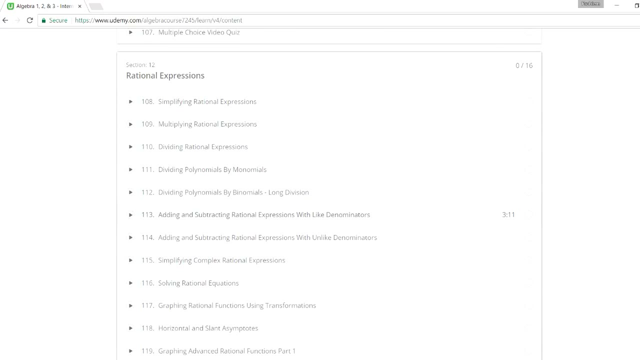 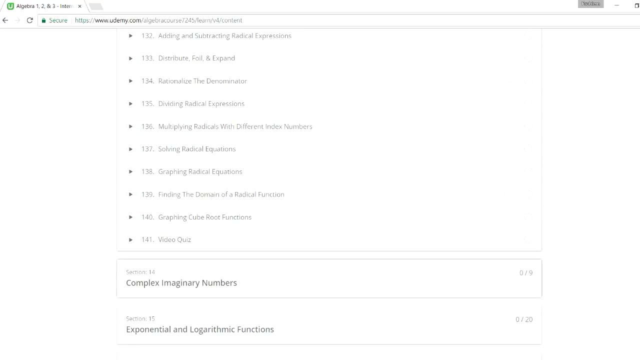 Next, quadratic equations: how to use a quadratic formula, how to graph them, how to convert between standard and vertex form. And then you have rational expressions And radical expressions, Solving radical equations, simplifying it, things like that, And every section has a quiz. 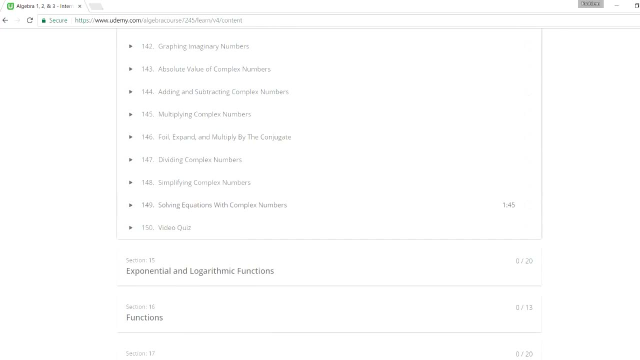 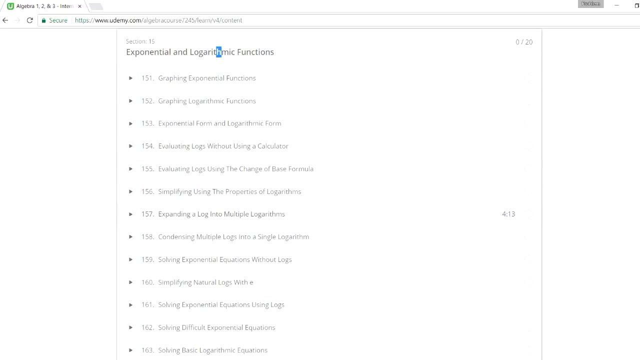 So you can always review what you've learned if you have a test the next day. So here we have complex imaginary numbers. You need to know how to simplify those Exponential functions. logs- I have a lot of videos on logs- And then this is just functions in general. 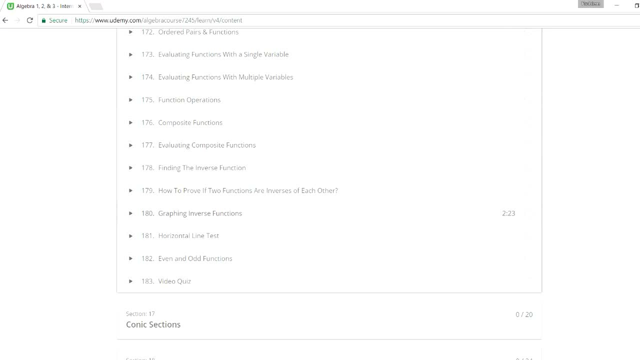 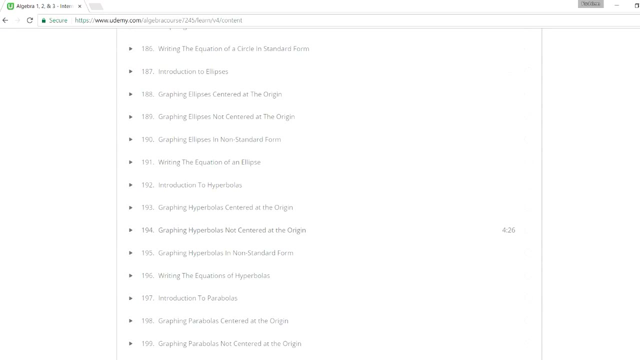 Vertical line tests, Horizontal line tests, How to tell if a function is even or odd, And then conic sections, Graph in circles, hyperbolas, ellipses, parabolas And things like that. There's two video quizzes. 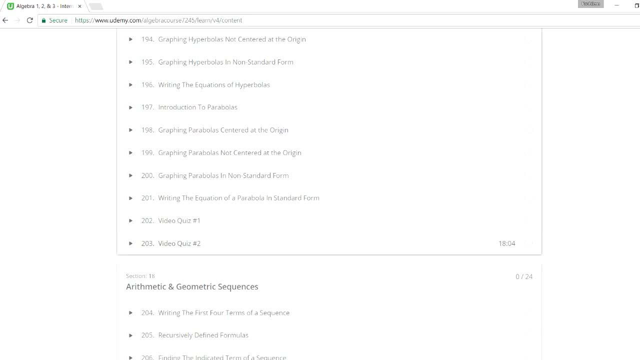 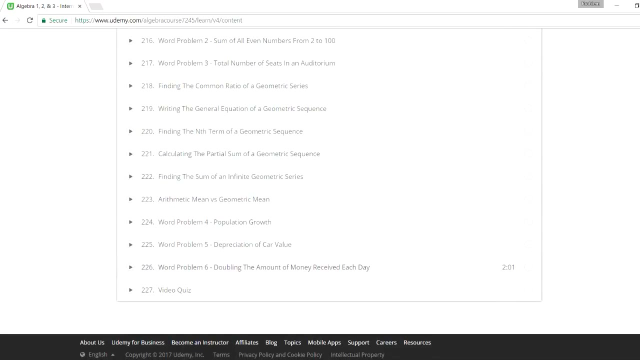 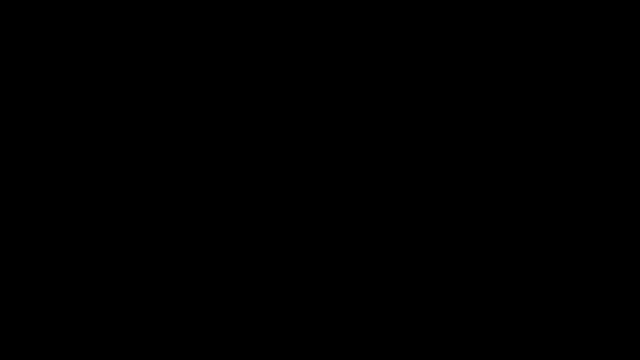 because it's actually a long section, And finally arithmetic and geometric sequences And series. So that's my algebra course, if you want to take a look at it And let me know what you think. Thanks for watching. I'll see you next time.